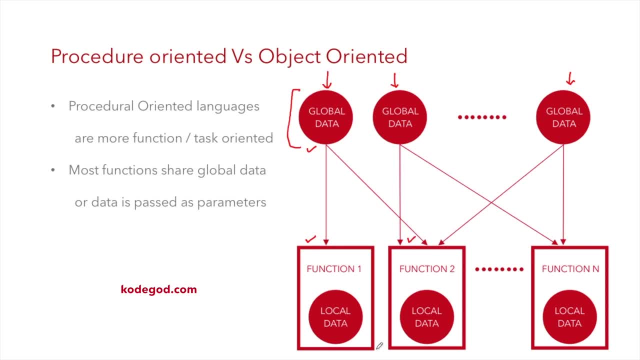 in other files. So again, not necessarily these are different files, So this can be a single file or multiple files as well. So important point that I'm trying to make over here is that global variable is accessible across all the functions. All these functions can access this. 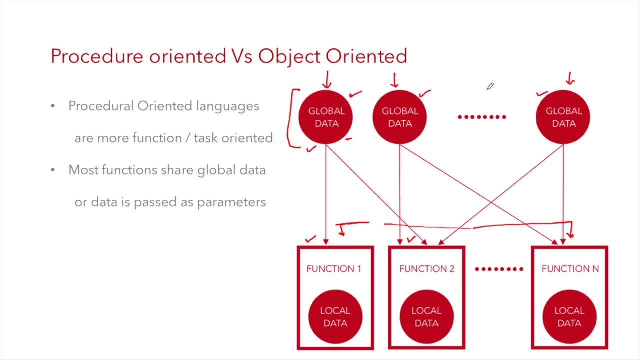 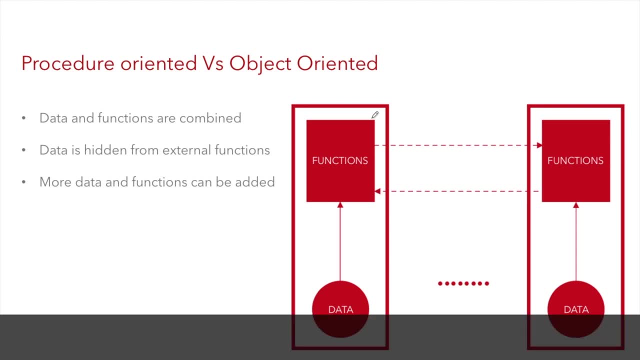 data, this data or this data. So in a way, there is no security, So any function is accessing anything. So now let us look at what object-oriented languages are offering us. So in case of object-oriented languages, data and functions are grouped together in these form of structures. 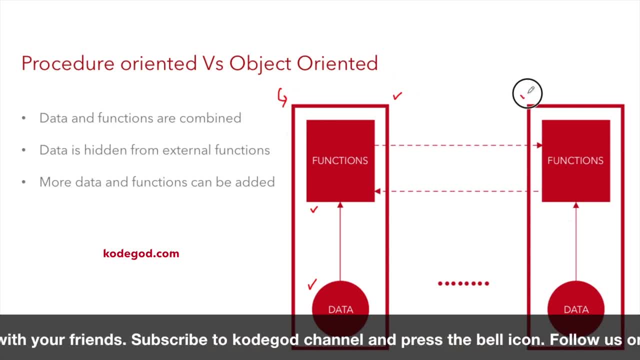 So let's say this is one structure, This is another structure. Let me call it as groups, because structure is something that we have already used in C, So let us not get confused with that term. So we are saying over here that functions and data are grouped together, So data is accessible from the functions of the same 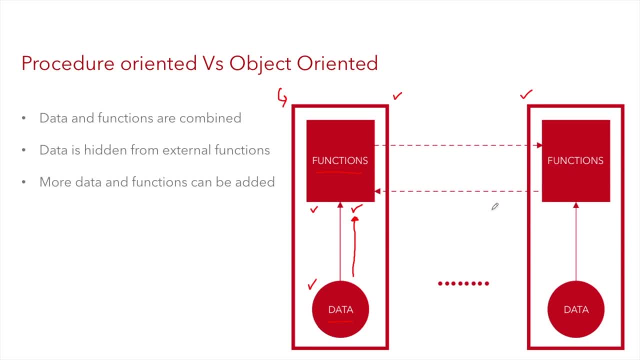 group. So outside functions cannot directly access the data. So this is not possible. So these functions or this group can access this data only if these functions are allowing it to do so. So this function can request or call these functions. These functions can. 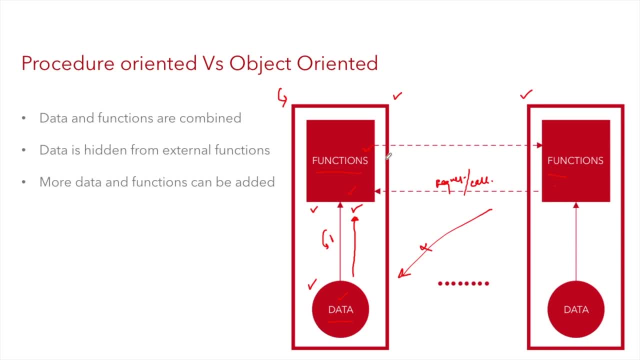 internally communicate with the data and then send output or response to these functions. So these functions can process local information And give output to the other functions, if these functions are called So. similarly, this data is not accessible directly by these functions. So, as we have seen, data becomes more secure in case of object-oriented programming. 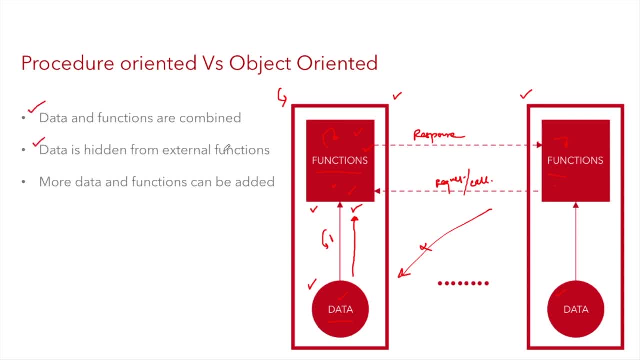 So data and functions are combined and data is hidden from external functions. And another important point is that more data and functions can be added. So, like this is my model 1. This is my model. 2. Subsequently, n number of models can be added. 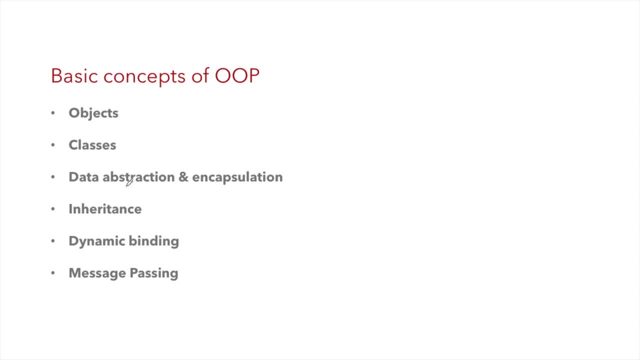 So moving on on the next topic, that is, what are the basic concepts of object-oriented programming? So these are very important features or concepts of object-oriented programming, Like objects, classes, data, abstraction, encapsulation. Irritance is one of the most important concept or feature provided by object-oriented programming. 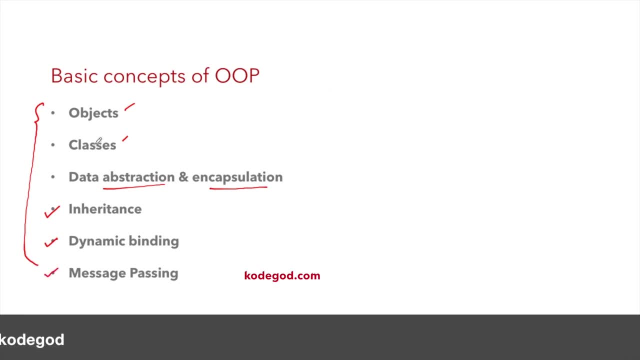 Data hiding- again as we discussed, and passage passing. So these are all important concepts. So, moving on on the next topic, that is, what are the basic concepts of object-oriented programming? These are the many different features we are going to discuss one by one. 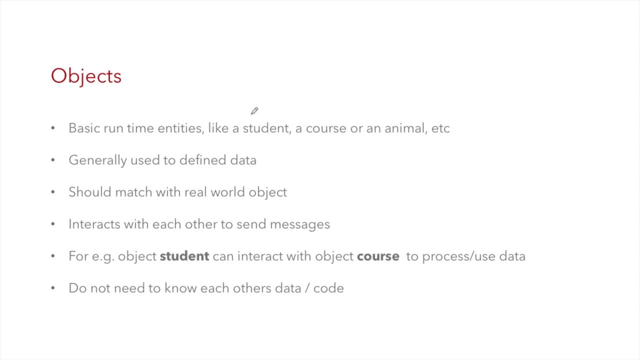 So let us start with objects first. So objects are basic runtime entities like student course or an animal, So these are usually real-world objects and they are generally used to define data And these objects interact with each other to send messages. For example, object students can be used to interact with object course to process or 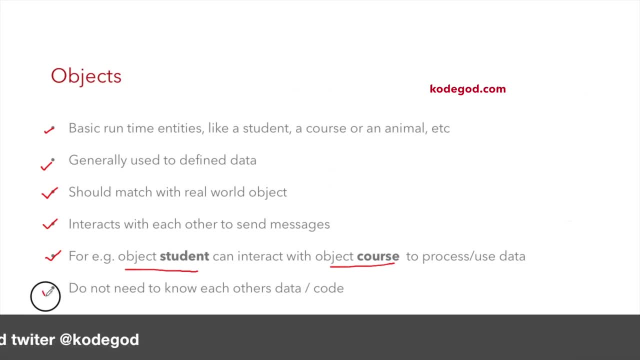 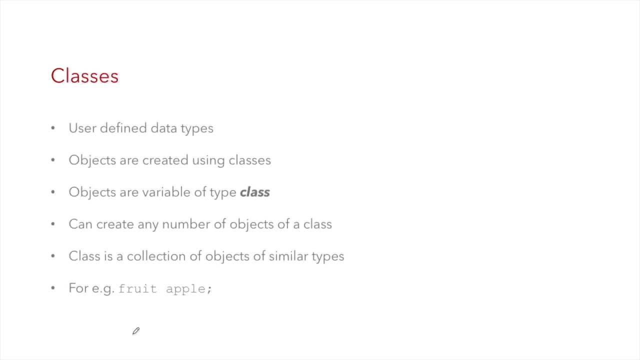 use data, not need to know each other's data. so, in case, i have object 1 and object 2, so they both do not need to know each other's data. now important question is how these objects are created. so objects are created using classes, which is next important feature provided by object oriented. 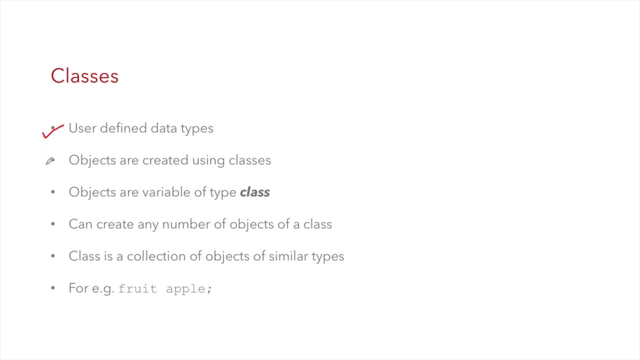 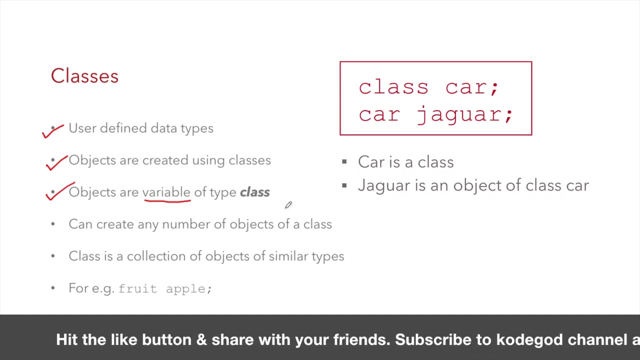 programming. so we discussed that classes are user defined data types and objects are created using classes. so in a way objects are variables of type class. so like we write in x, so x is a variable of type integer. so when i have a class called as car, then jaguar becomes an object of type class having. 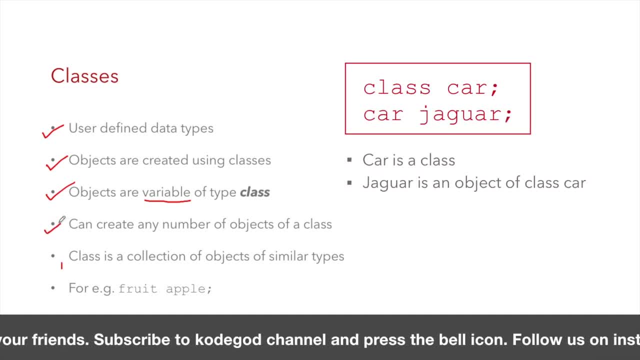 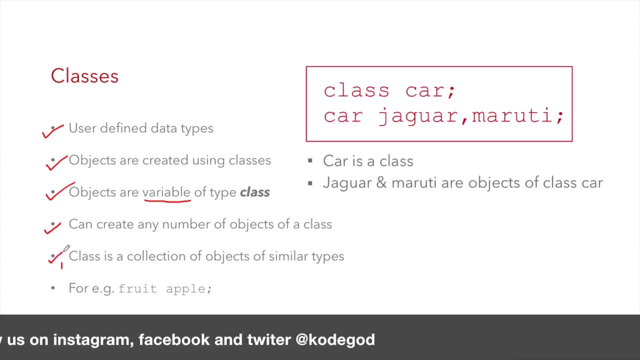 name car and when we create a class we can create any number of objects of that class. so classes is a collection of similar data types. when i say car jaguar or car car maruti, so maruti and jaguar are objects or similar objects of class car. so another example is: 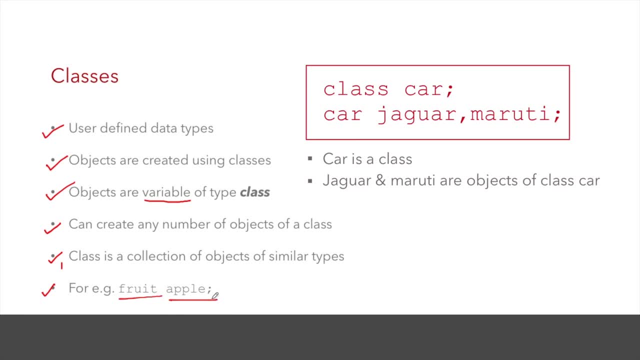 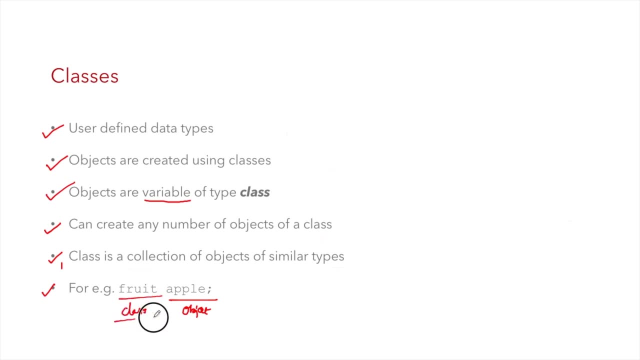 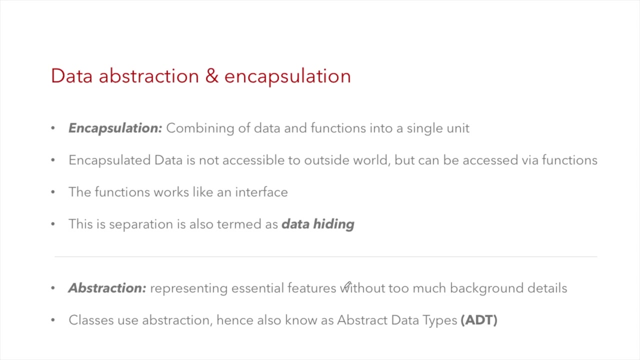 let's say fruit is a class and then apple is object of class- fruit. so similarly, we can have fruit as class and then we have, let's say, apple, then banana or let's say mango. so all in these three are objects and fruit is a class. another important feature is data abstraction and encapsulation. 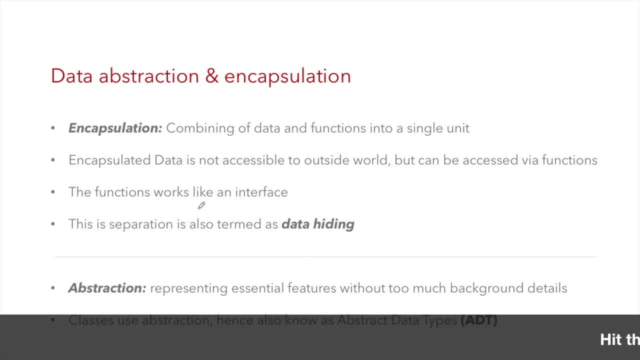 so encapsulation is nothing but combining of data and functions into a single unit. so, as we discussed earlier, data and functions can be combined together, which forms a single unit, which is called as a class. so data and functions can be combined together, which forms a single unit, which is called as a class. so 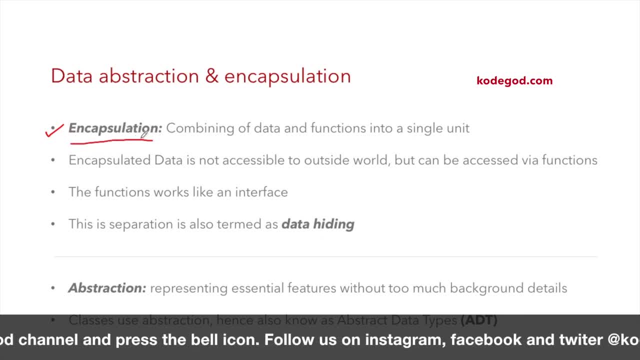 this feature is known as encapsulation, so binding of data and functions together, or combining of data and functions together, is called as encapsulation. next point is encapsulated data is not accessible to the outside world, but can be accessed via functions. so when i have a single unit class, 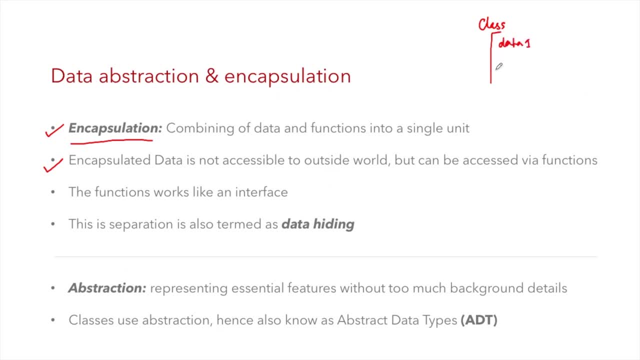 so data one, data two, so these are two data variables of that class. then is the food function saying that we can have these two functions? then i have function one, function two, these two functions. so this in total is forming a single unit. we are calling it as: 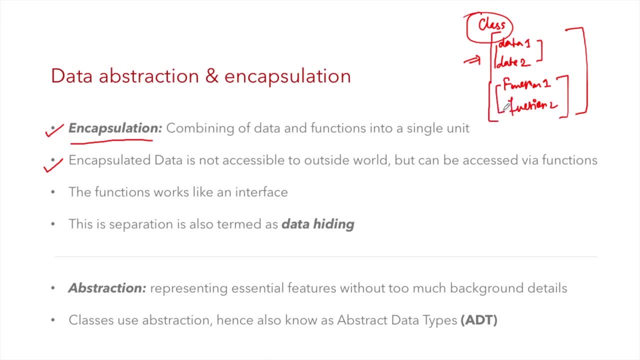 class and this data is not accessible to the outside world, but it can be only access via these functions. so in a way, these functions works like an interface, so in order to access the data- and this separation also provides us security and hence the term is known as data hiding- 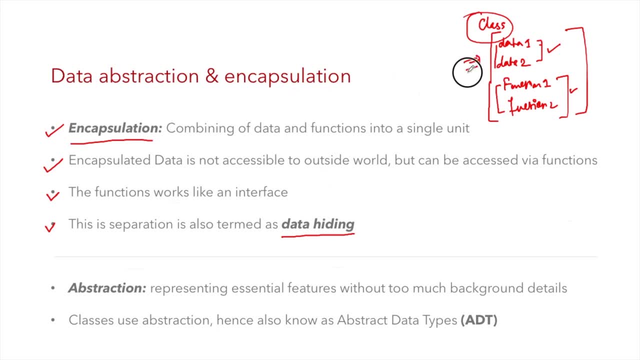 because we are hiding this data from outside world. so next feature is abstraction, and abstraction is nothing but representing essential features without too much background details. for example, if i have a class, so let us say i have a group called as car, then i will just have attributes or features of that car, as, let's say, number of wheels. 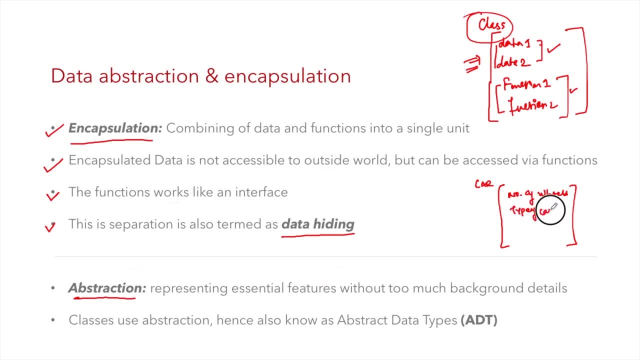 then type of car, okay, and so on. so i'll be using only essential features. i'll not be adding too much of the background details. i can create my own classes or these custom data types without too much of background details. so classes use abstraction. hence classes are also known as abstract data types or adt in. 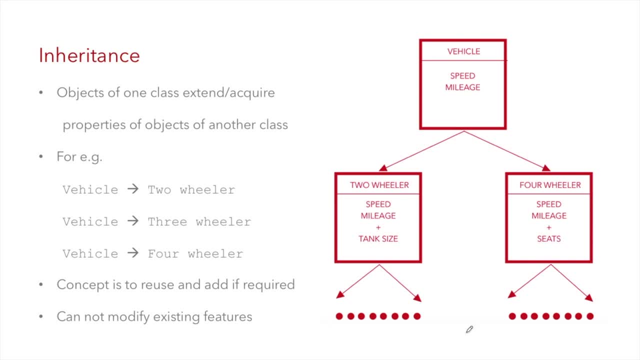 short form. now one of the most important topic is inheritance. inheritance allows objects in your program to extend or acquire properties of objects of another class. so let us try to understand this via an example. let us assume i have a class vehicle and then i have data members as speed and mileage. so this is my base class and i'm going to create one more. 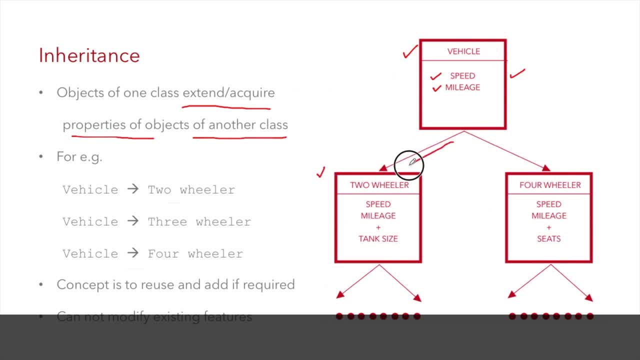 class wherein i am inheriting or acquiring information from this base class, which is mileage and speed plus, i'm adding my additional information, okay, and i'm calling it as two wheeler. similarly, i have four wheeler as a class name and i'm again inheriting information from the class vehicle and this is 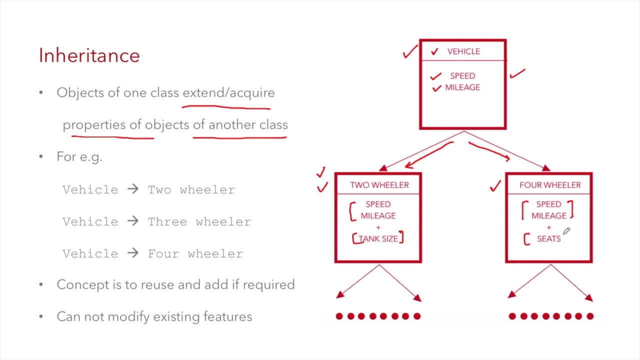 inherited information: speed and mileage, plus. i'm adding seats or number of seats as additional data. member in the class four wheeler: okay. similarly, these can be further inherited too. okay. so this is our example. so vehicle is the base class and we have inherited properties from that class to 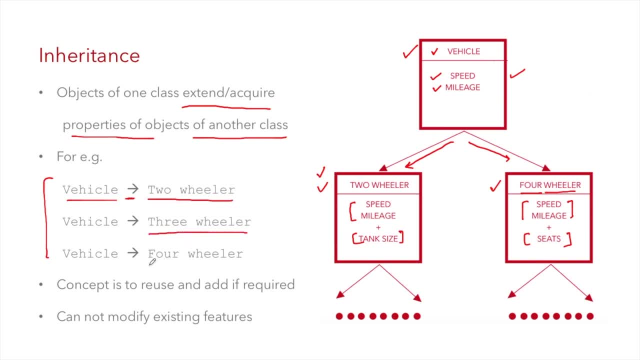 class two wheeler, similarly three wheeler, four wheeler and so on. so the concept here is to reuse and add if required, because we are reusing the code. it will save our job on creating the same variables again and again. it will save a lot of memory as well. it will save a lot of development. 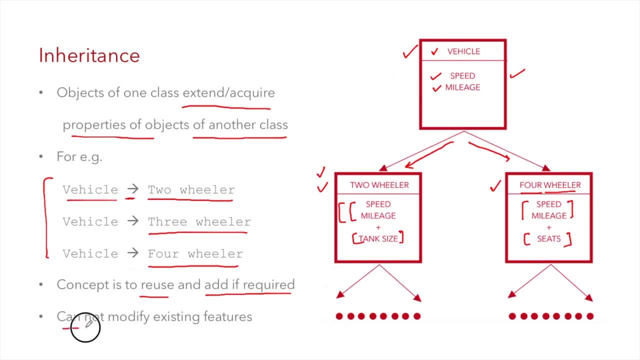 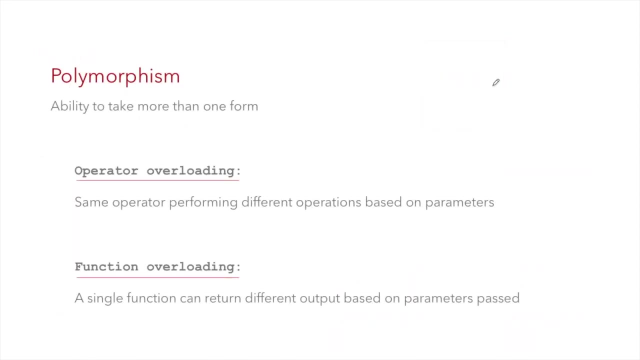 time as well. most important thing about inheritance: that we cannot modify existing features, as in, we cannot modify properties of my base class, so i cannot go on and modify this variable name or or delete these data members now. next is polymorphism. polymorphism is ability to take. 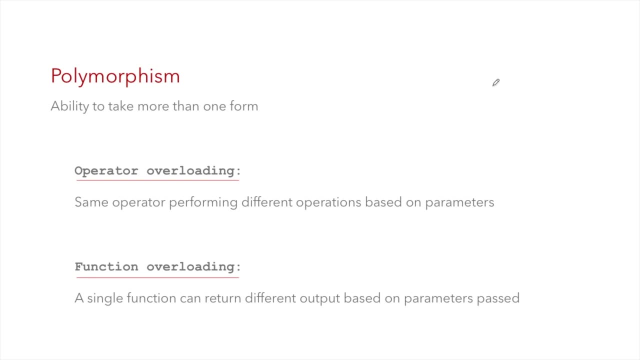 more than one form or it gives multiple meanings to the same thing. so two important features in c++ are, or in object oriented programming are object oriented programming, and object oriented programming and object oriented programming are operator overloading and function overloading, so same operator can do two or more different. 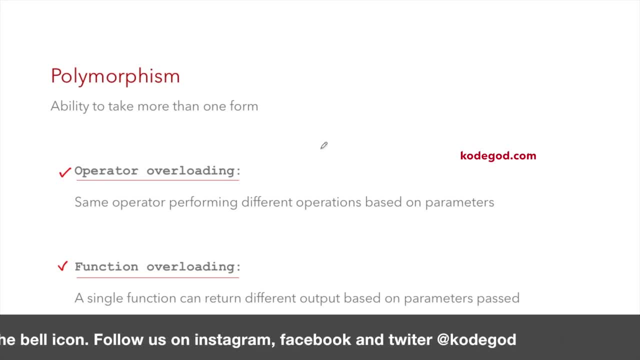 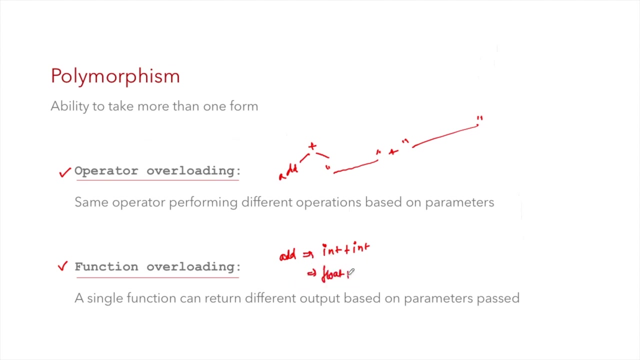 operations, that is, operator overloading. so here let's say plus sign can either perform addition or plus sign can. you can be used to concatenate two strings. similarly in function overloading we can use function add to add to integers, or it can be used to add two floats. so in function overloading single function. 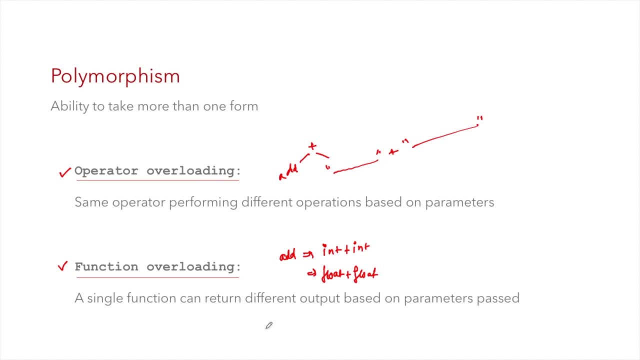 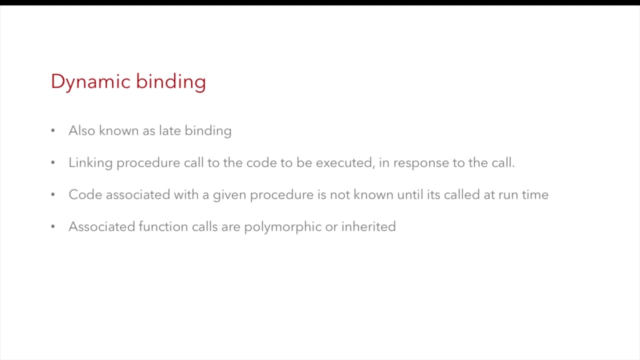 so in function overloading, single function can return different output based on type of parameters which are passed to that function. so very important topic. we are going to touch these topics again in Next important point is dynamic binding. it is also known as late binding. Dynamic binding is nothing but linking of procedure call to the code to be executed in response to the call. 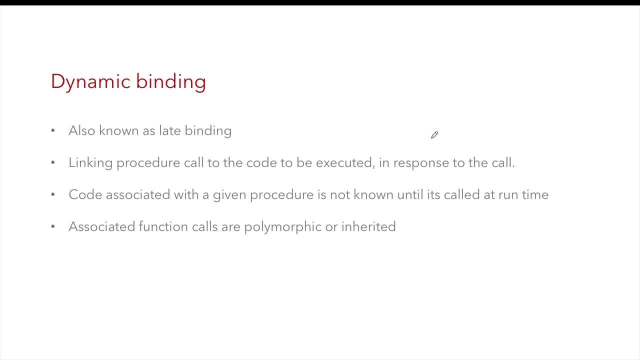 So complex statement. let me try to simplify it here. Suppose we have class xyz and it has function associated with it as function1. So when we create this object, at the run time when this function is called along with the object name, So at the run time associated call or the definition of this function will be called. 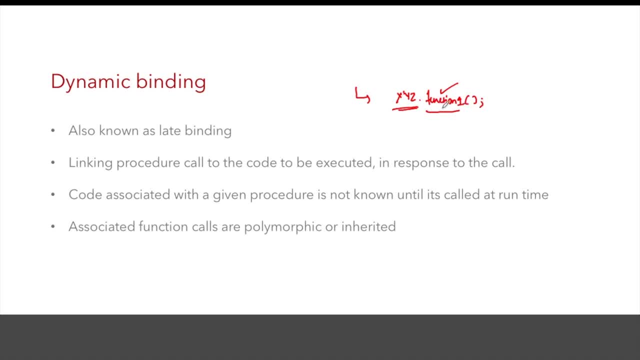 So in a way this becomes a dynamic binding. so this binding is done at the run time. Now you may claim that xyz is already created object, but at the run time you can create n number of objects, right? So let's say, you create xyz and xyz is already created object. 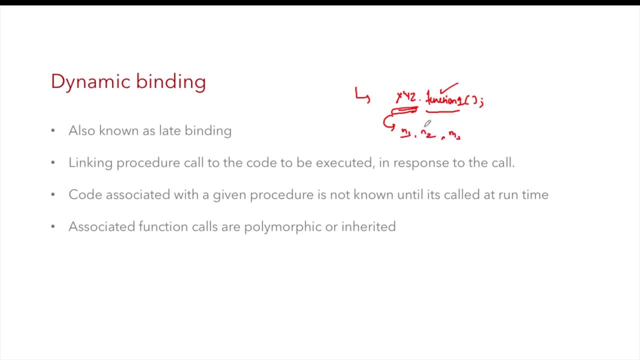 You can create multiple copies: n1,, n2, n3 and so on. So all these technically can still call this function. Because these objects are created at run time. binding is also done at the run time dynamically. Another important thing is that code associated with the given procedure is not known until it is called at the run time. 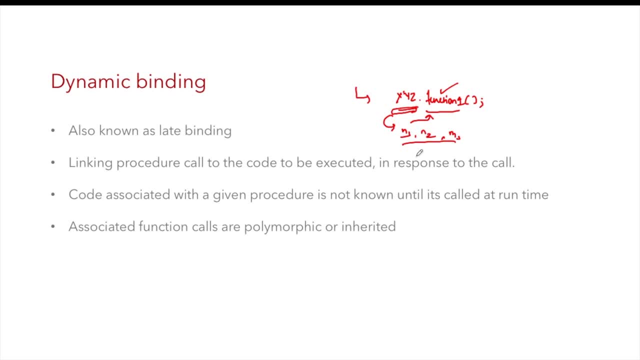 The reason is also that associated functions are sometimes polymorphic or iterated. Again to simplify it: when we say polymorphic, that is either we have function overloading Or operator overloading. So at the time of execution, compiler will make a call. that call is referred to which function. 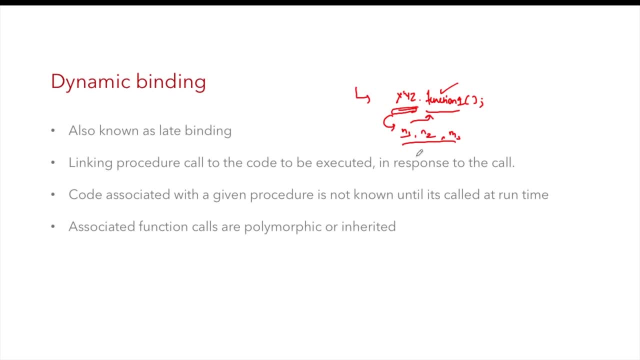 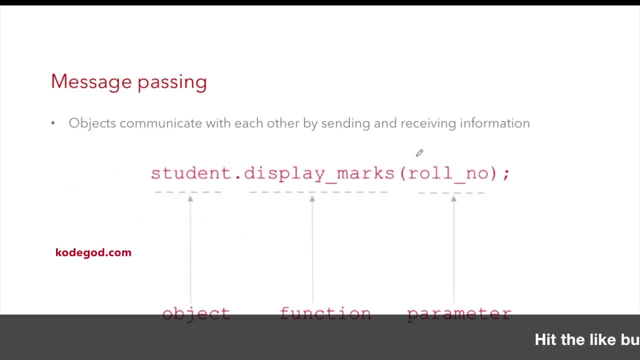 Similarly, function can be iterated. hence calls can be decided at the run time by the compiler. And because objects will be created at the run time, even in the case of polymorphic or iterated functions, There would be a dynamic binding. Now the last important topic is message passing. 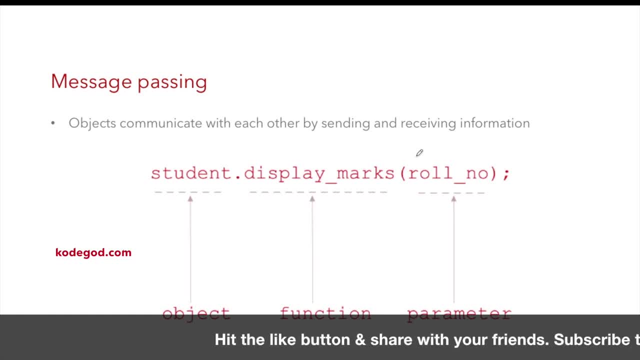 In object oriented programming, objects communicate with each other By sending or receiving information using parameters. So let's say student is my object, Then display marks is a function And then role number is a parameter. So this parameter is sent from the called function and is received at the called function. 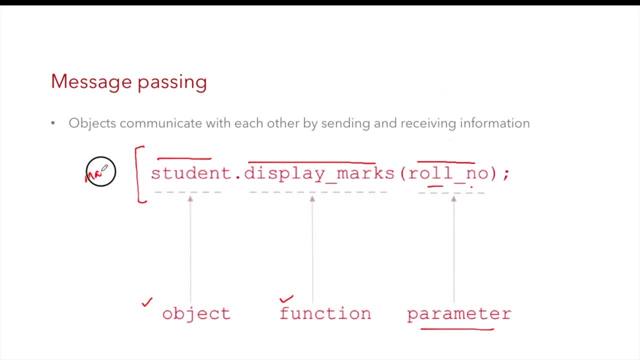 So if this code is inside of your main function Or any other function, So this function is sending this parameter And this function will be receiving this variable. So this is how message passing plays critical role in object oriented programming. Now let us look at benefits of object oriented programming. 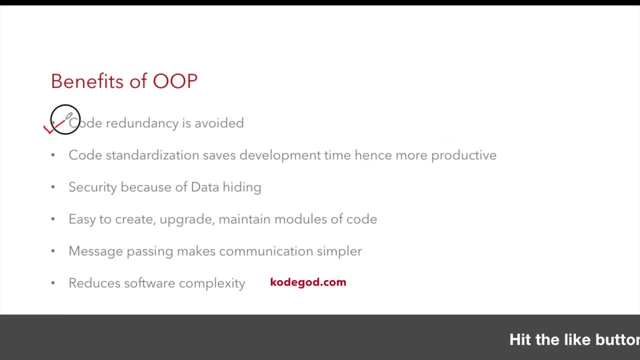 Because of the features that we have seen earlier, Code redundancy gets avoided very nicely. There is very less redundancy in the code Because of code standardization. Development time is saved And hence development becomes more productive. Because of feature of data hiding, Object oriented programming provides good amount of security. 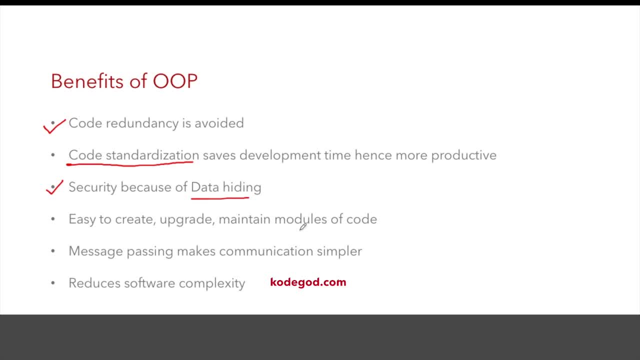 Models of code are easy to create, upgrade and maintain. In object oriented programming We have seen message passing makes communication very simple. Because of the overall features that we have seen so far, We can say that it reduces software complexity Because of features like inheritance, where we reuse the code. 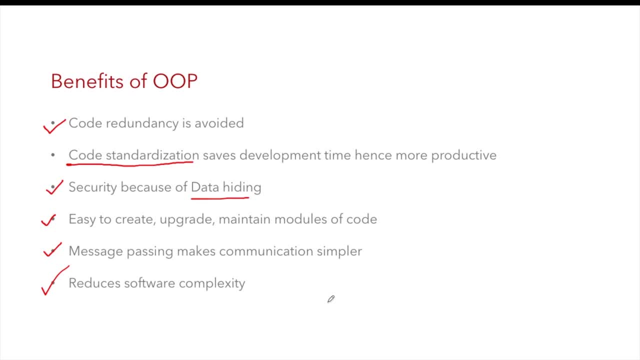 Or feature of polymorphism, Where we can have multiple meaning of a same function. Now, before we begin with actual objects and classes, Let us spend some time on how input and output can be carried out in C++. So we have two operators to do this job. One is right shift operator. 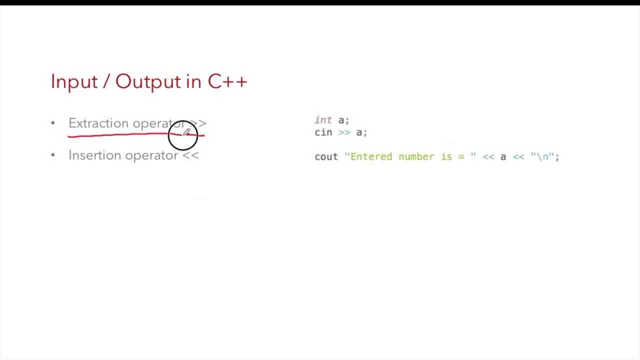 In case of inputting, we refer the same operator as Extraction operator And then we have insertion operator, Which is left shift operator. So here is one example: I say int a semicolon, Then cin, extraction operator a. So whatever value that I am going to enter will be stored in the variable a. 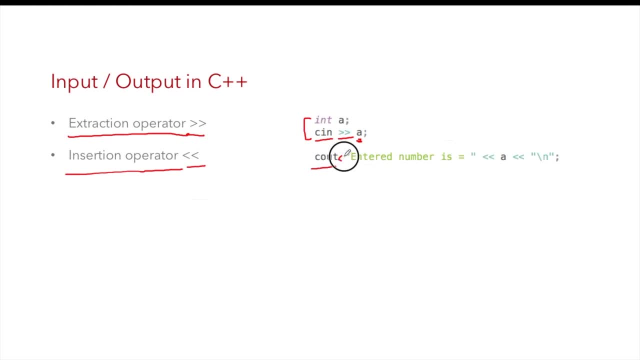 Then I have cout. I will be using my insertion operator over here. So cout, insertion operator, My string enter number is equal to, Then again one insertion operator And I am providing value of a. So whatever value of a that is entered at this tape, Let us say 10- 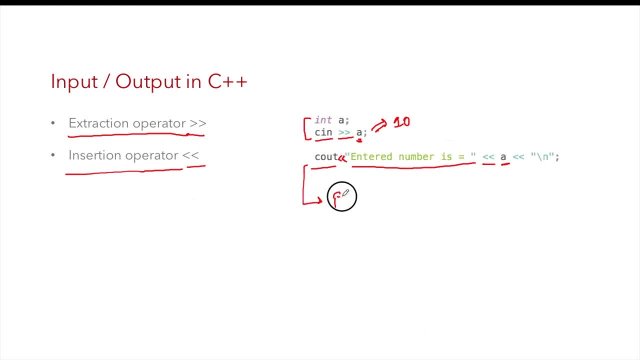 So output of this statement would be Entered. number is equal to 10 And we know that slash in is a white space character Which will take cursor to the next time From this line. it will come to this line. So cin and cout is something that we will be using commonly. 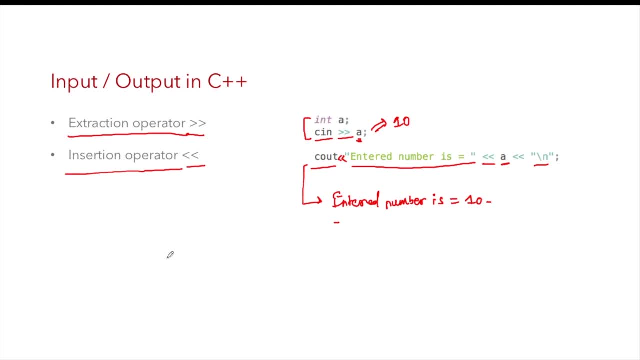 It is almost a replacement to our printf and scanf statement. Now let us touch back the topic of polymorphism. As we have seen, polymorphism gives different meaning to the same operation, Depending on the context. For example, we know this operator, which is multiplication operator. However, in c, 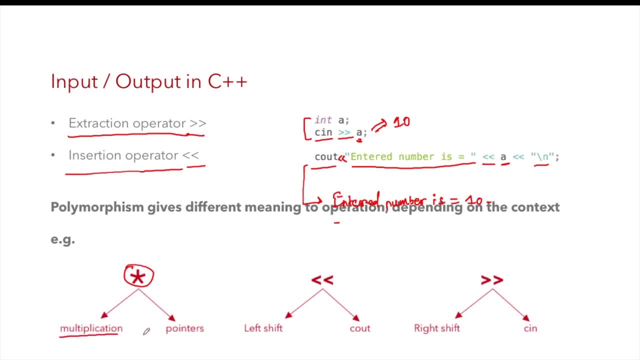 However, in c language also We have used it as multiplication Plus. we have used for pointers too. So in a way c language also had this polymorphism feature. Now, in case of input output operator, We know that this is a left shift operator, Which was a bitwise operator in c. 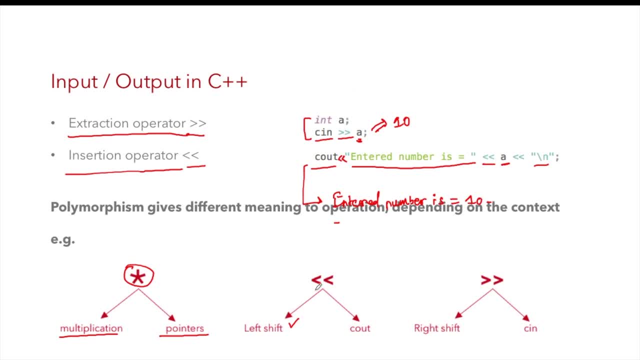 It is still a bitwise operator in c++ But, depending on the context, when I use cout It works as Insertion operator. Similarly, This is our right shift operator in c and c++. However, when we use it In conjunction with cin, It works as extraction operator. So simple enough. 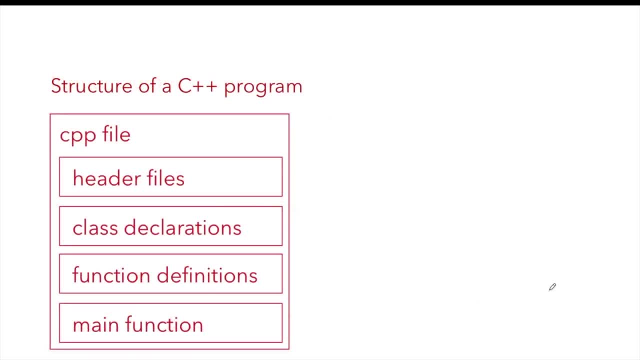 Finally, we will just check What is the structure of a c++ program. So here we have a c++ file, Then We Start with header files, Then we have our one or more class declarations, Then we can have multiple functions, That is, one or more function definitions, And after that, finally, we have our main function.